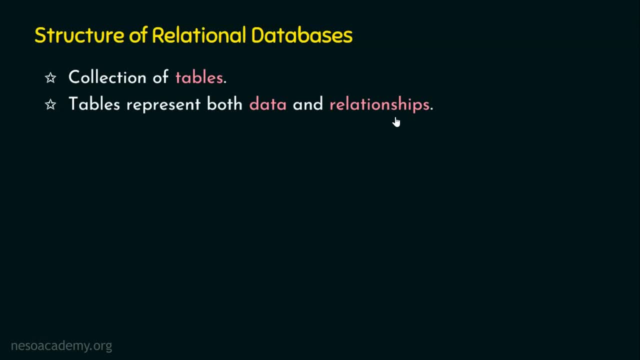 Mohammed Khan is having the roll number 101 or 101.. So what does it mean? This means there exists a relationship among the values that are stored in the table. In other words, when you have a row, each value in a row is having relationship among other values. 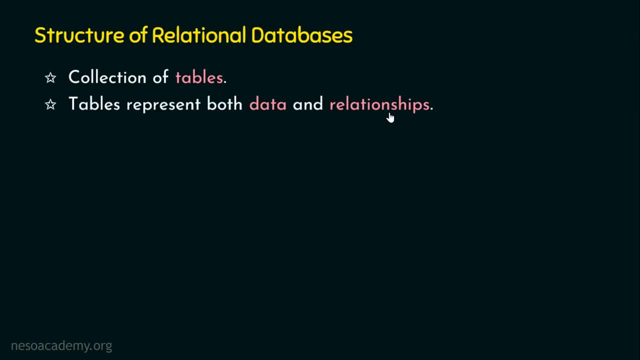 And not only this. tables can also be used to maintain the relationship among other tables. Say, for example, an advisor table can be used to maintain the relationship between a student table and an instructor table. No worries, I will explain that shortly, And that's why I have 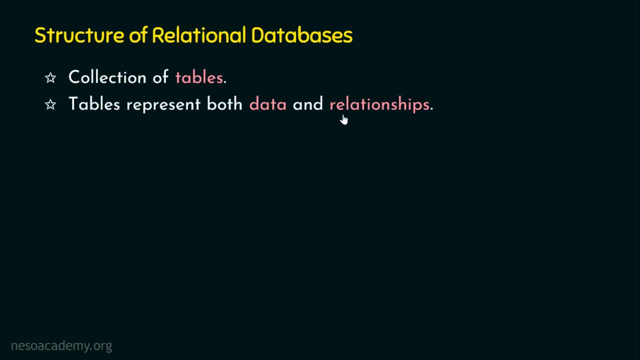 mentioned here as tables represent both the data and the relationship among the data present in the table. Now, in relational model, are we going to refer this as table? No, we are going to refer this as relation. Then why the term we are using for representing tables? 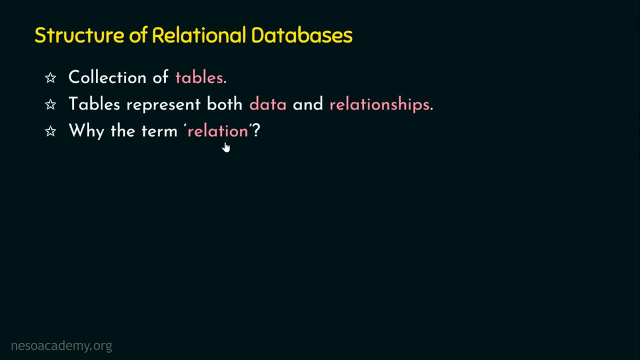 as relation in relational model, Because there is a close association between the DBMS concept- the table- and the mathematical concept- the relation, And that's why in relational model we use the term relation instead of referring it as tables. Anyway, we will talk about this. 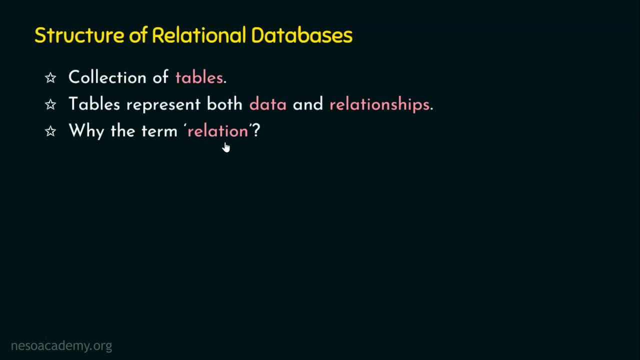 elaborately in the coming video. So let's get started In the coming lectures. for now, just understand: a table in relational model or a table in relational databases are referred as relation. Basically, relations are tables, but the important thing to note here is it has a very close association with the mathematical concept. 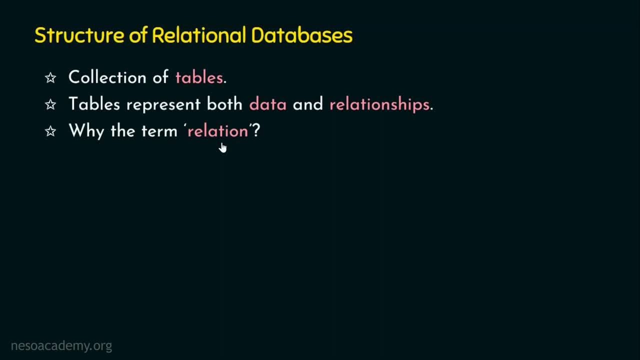 called relations. Anyway, you will understand about this when we see the concepts relational algebra and relational calculus in the coming lectures. For now, just understand: a relation in system is basically a table only, But we can apply many mathematical operations on relations. when you compare with the table, Then what about the rows and columns? 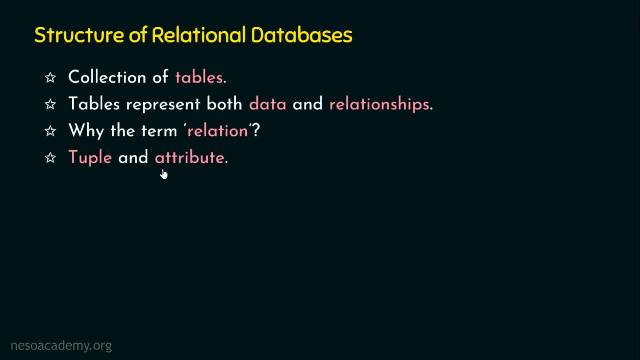 A row in a relation is referred as tuple and a column in a relation is referred as attribute. In a table, we represent rows and columns In relation. we represent it as tuple and attributes. Remember, a tuple is basically a row in a relation and, coming to attribute, this is: 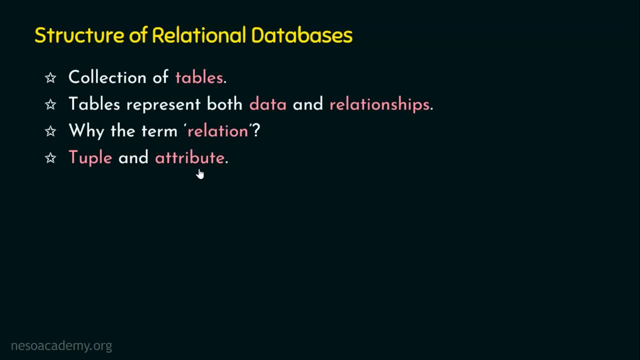 the column in a relational database management system, And we have already talked about instances and schemas. What is an instance? The data present in the database at a particular moment. we call it as an instance. In relational database, we call it as relation instance. 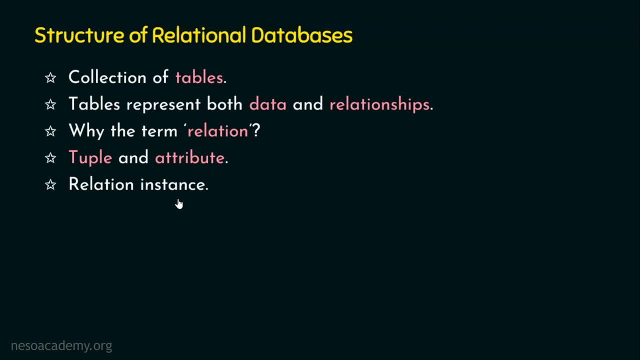 What do we mean by this? This relation instance refers to a specific instance of a relation. It means a specific set of rows. For example, if you are referring to a specific set of rows in a relation, then this is referred as relation instance. 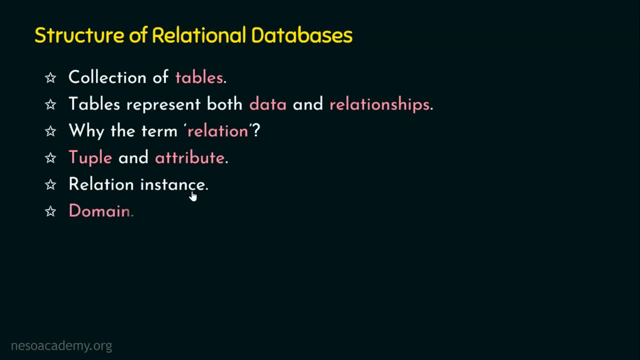 And coming to the next important concept in relational database, which is the domain. What is a domain? It is actually a set of permitted values. I'll give you an example. Let's take we are talking about a banking database and let's assume this banking database is a. 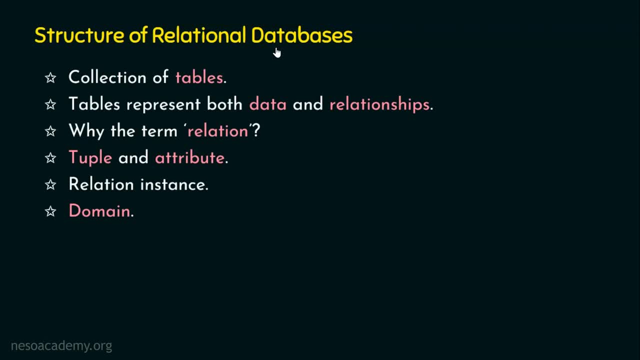 relational database. Let's also assume this bank has five branches, only five branches. The branches are in New York, Washington, San Francisco, Chicago and Austin, Or whenever we see a value in the database against a branch, then only these five values are permitted. 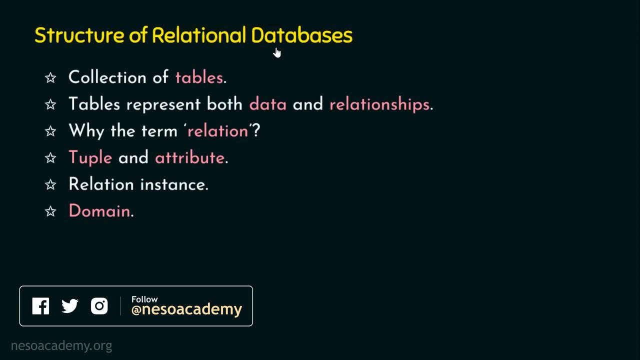 What are the values? New York, Washington, San Francisco, Chicago and Austin? Let's say someone is trying to insert a row into the table with the value Los Angeles. Obviously, Los Angeles is not a set of permitted values, because there is no branch called Los Angeles. 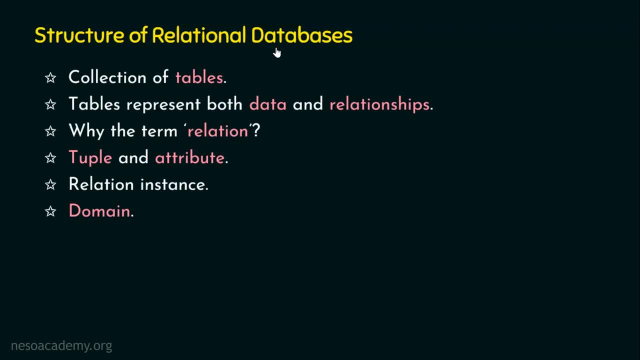 for that particular bank. In that case, that particular value is not belonging to a set of values, Right? So that is what we call a set of permitted values, And that is what we call a set of permitted values, And that is what we call a set of permitted values, And that is what we call a set. 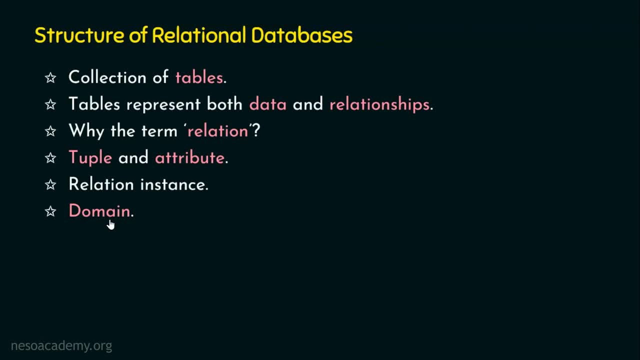 as a domain. Basically, a domain is a set of per meter values, and please see here an important question: when a domain is said to be atomic? The answer to this question should be known by all database administrators, because this is going to be playing a crucial role. 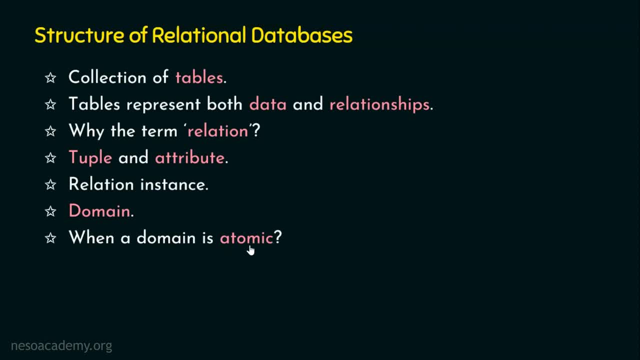 in relational databases. So let's understand what do you mean by atomic. A domain is said to be atomic if the elements in the domain are considered to be indivisible. Let's say we have a column in the table as the phone number. This phone number, if it is considered 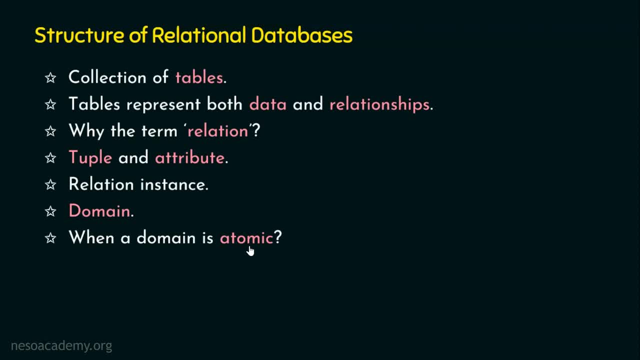 as a single value, then it is an indivisible unit and we can say that this phone number is atomic in nature. Instead, if we consider phone number has multiple units like country code, area code and the local number. In that case, this phone number is referred as nonatomic. 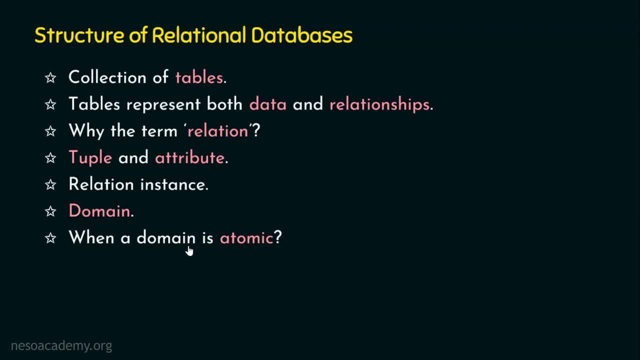 So please be noted that when a domain is said to be atomic in nature, when the elements of the domain are considered to be indivisible. Subtitles by Jai Jairoo. So in the domain example we have taken branch name right. 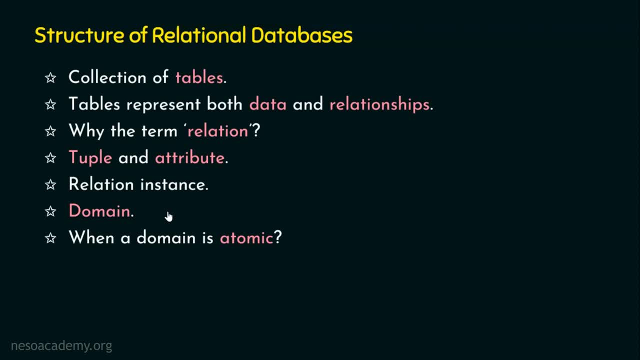 The branch name that we have taken are New York City, Washington, San Francisco, Chicago and Austin. All these are indivisible in nature, So we can quote that the values present in the branch name is atomic in nature because it cannot be divided further. 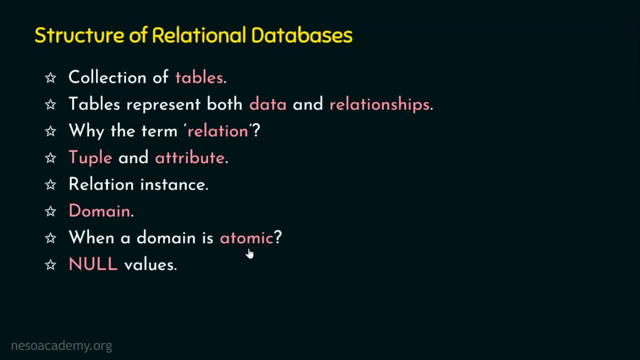 And another important thing to note about the relational database is this: null values. What is a null value? Remember this. null value is not a blank value or empty spaces, or no value or no characters. Null values in DBMS is a special value which represents that the value is either unknown or that does not exist. 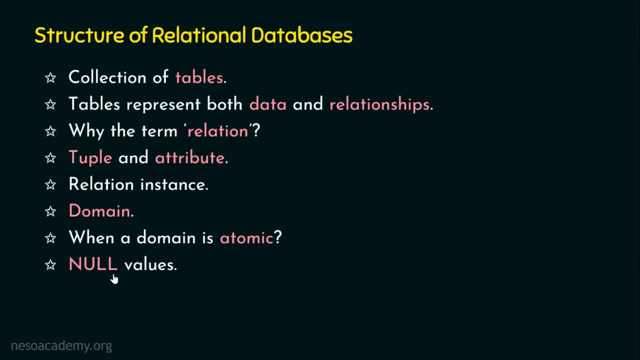 I'll give you an example. Let's take if a student has no phone number. In that case, we cannot give 0 as the phone number, because 0 is not a null value. At the same time, it may be added in the future. 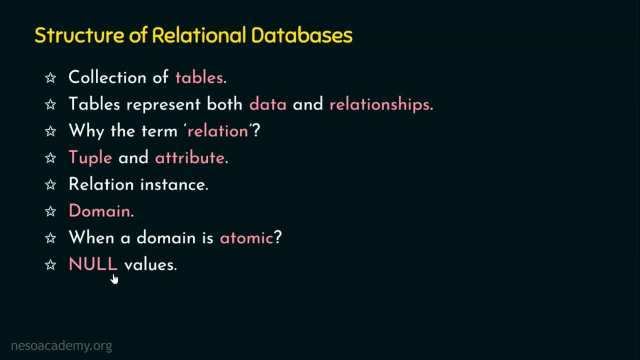 So a student who is not having a phone number In the database, the phone number column. for that particular student it should be a null value because it is either unknown or does not exist. I will elaborate about the concept of null values when the course progresses. 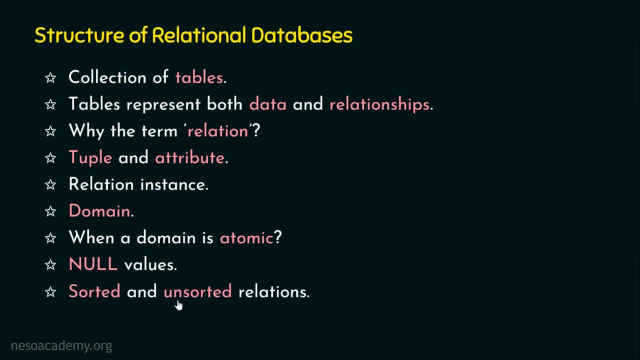 And I'll ask you a question: Will. the relations are generally sorted in nature or unsorted in nature? The relations are generally unsorted in nature. The reason for this I'll explain you in the following slides. Let's take an example: relation. 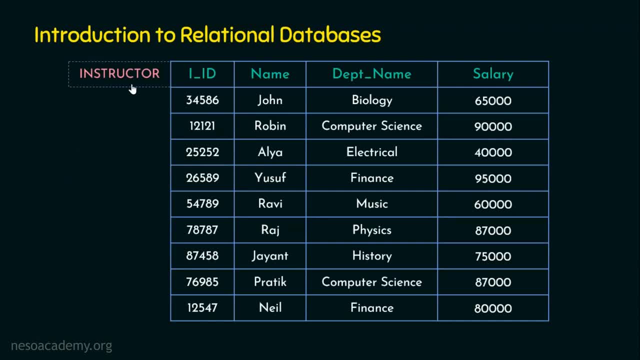 The example we are going to take here is the instructor relation, which contains four attributes: Instructor ID, Instructor Name, Department Name and Salary. And can you see here we have some rows here. This is actually a tuple in relational database 3,, 4,, 5,, 8,, 6.. 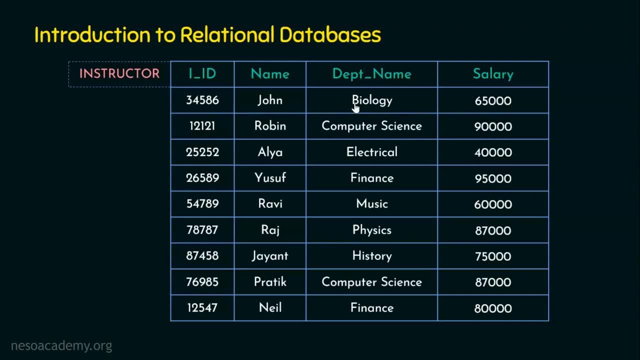 The instructor ID is pertaining to John, who is working for the Department Biology, who is drawing a salary of 65,000.. Now the instructor ID of John is 3, 4,, 5,, 8, 6.. And 3,, 4,, 5,, 8, 6.. 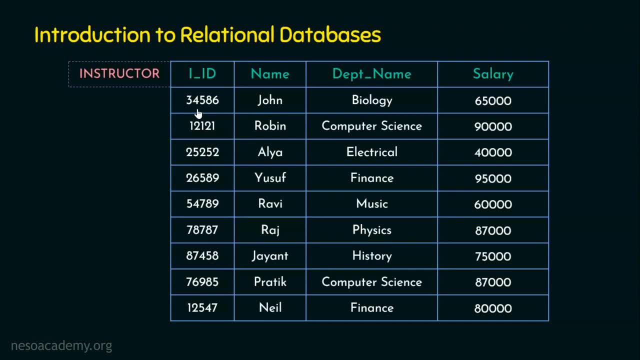 is actually John, And that's why I told you a row in a table or a tuple in a relation represents the relationship among a set of values, And this is about the instructor relation. I'll show you one more relation: the student relation. 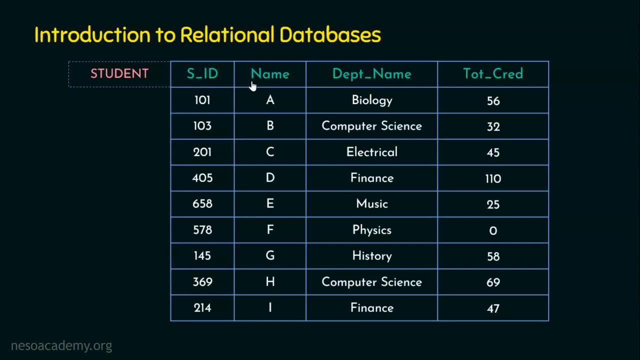 In the student relation we have four attributes: Student ID, Student Name, Student Department and the total credits earned by the student. So far we have seen two relations: instructor relation and student relation. Let's assume these two relations are a part of university database. 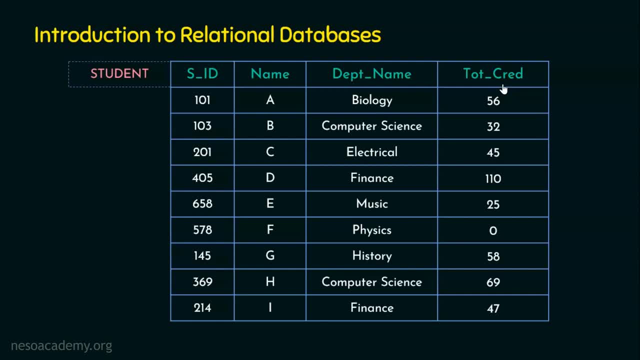 What is a database? It's a collection of table. In this case we are assuming student table or student relation and instructor relation are part of university database. How the relationship between the tables or relations are established, It is also achieved using another relation. 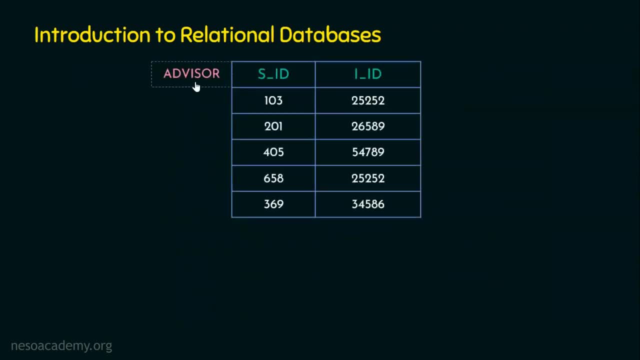 I'll show you that now. In this case, we can see that the advisor is a relation that contains exactly two columns: the student ID and the instructor ID. The advisor for the student who is having the student ID 103 is 25252.. 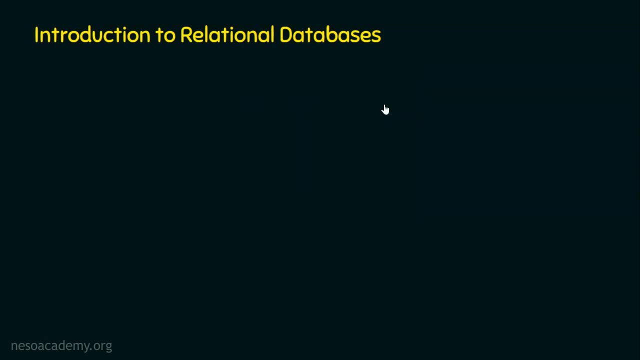 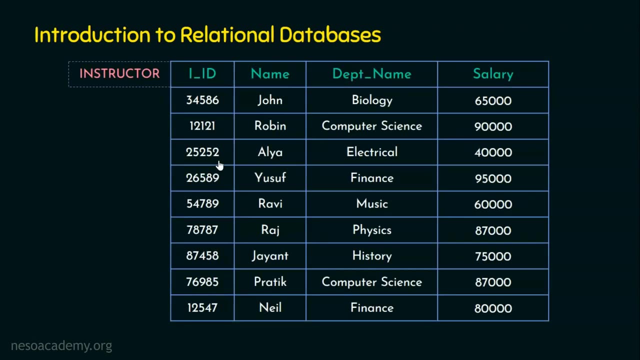 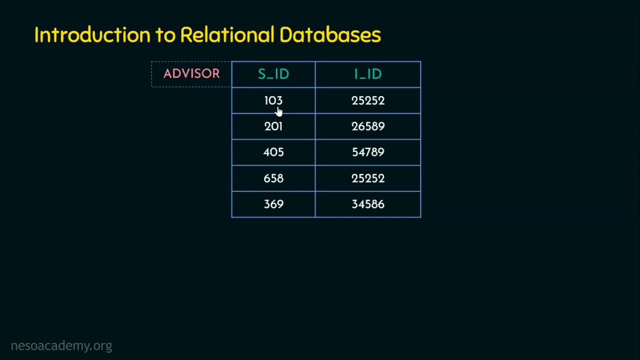 What do we mean by this? It means- I'll go to the previous slide- 103 is B and the instructor for the student B is Alia 25252.. That is what is mentioned here. The student with the student ID 103 is B and the student B's advisor is Alia, who is having the instructor ID 25252.. 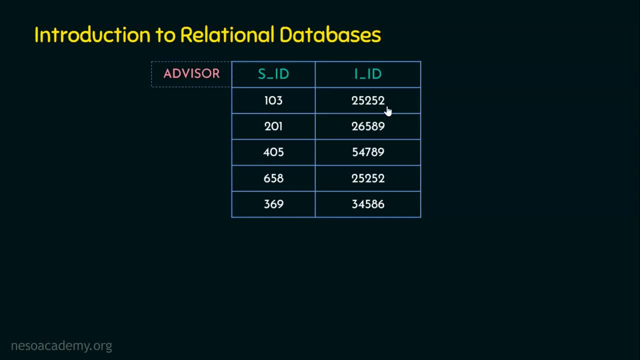 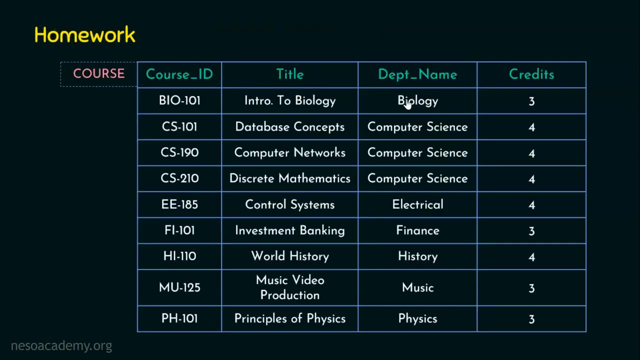 And this is how the relationship among multiple tables or relations are maintained in the relational database management system. Before we sign out, let's see a homework question. Here is the course relation. This course relation has course ID, the title, the department name and credits. 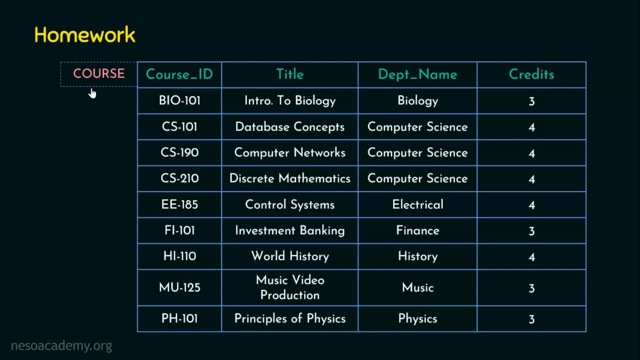 And what I am asking you to do is just try to figure out the relationship between the student relation or the instructor relation with this course relation. So this will definitely help you How these relationships are maintained in the database. Also, I am going to answer you one more question.